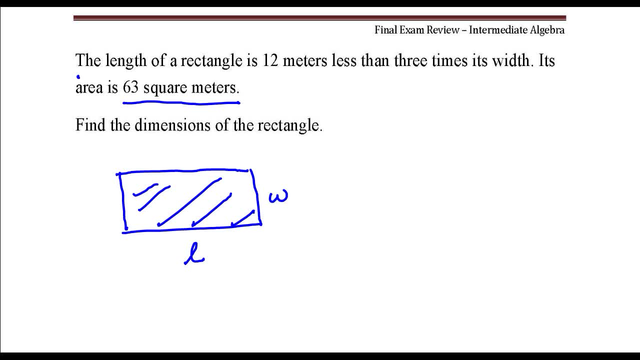 If you look at the very first sentence, it says: the length of a rectangle is 12 meters less than 3 times its width. Okay, so this length, L is that word is. is that equal sign? 12 meters less than 3 times its width. 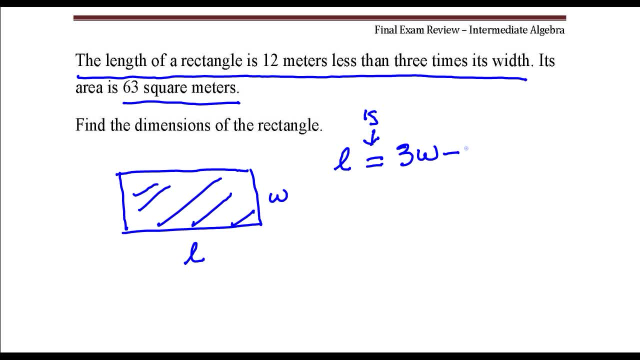 So 3W minus 12.. Okay, And we also know that the area of a rectangle is length times width, and in this case the area is 63 square meters. so I'm just going to replace A with 63, and I'm going to replace this L with 3W minus 12.. 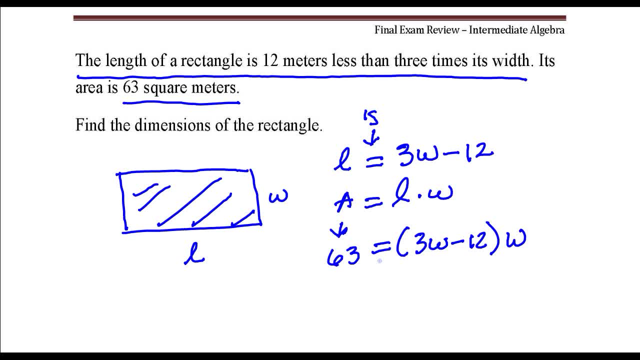 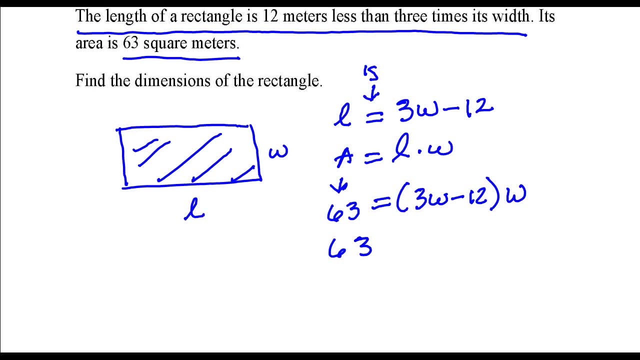 Okay, Okay, Okay, Okay Okay. That's length times. width is equal to 63 square meters. Okay, so I'm just going to multiply this out: 63 is W times 3W, that's 3W squared, and W times a negative 12,, that's minus 12W. 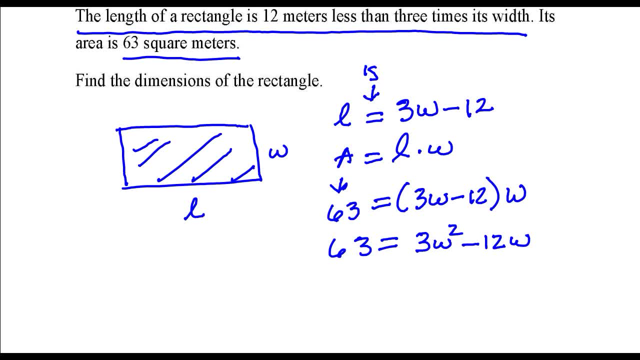 This equation is quadratic, so what I want to do is I want to get all the terms on one side And then I want to get a zero on the other side of the equation. so I have 3W squared minus 12W, minus 63, because I subtract 63 from both sides of this equation and the other side is going to be equal to zero. 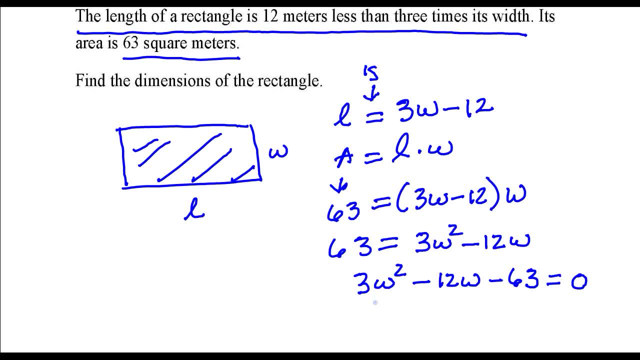 Okay, so to solve this quadratic equation, I want to factor this: It's easier if you factor a 3 out of E. It's easier if you factor a 3 out of E. It's easier if you factor a 3 out of E. 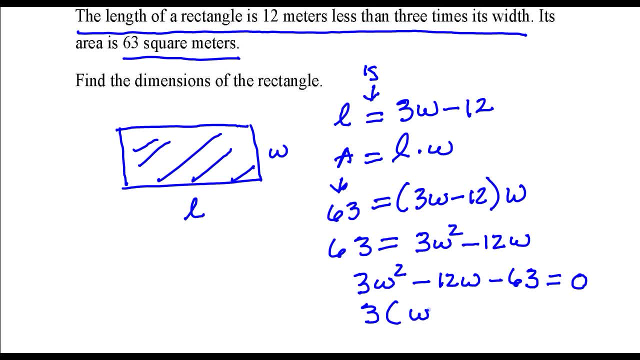 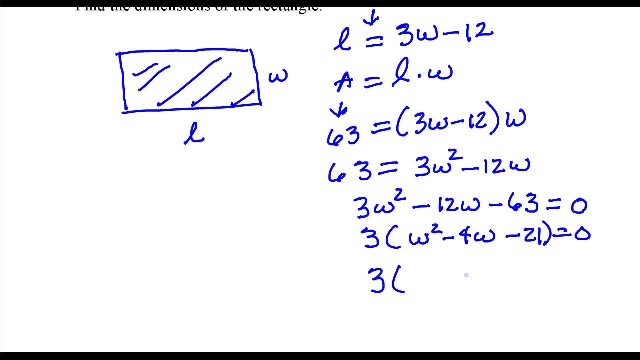 And then we'll write this quadratic expression as a product of two binomials. So I'm looking for two numbers multiplied together, that's negative 21. And then I'm going to write this quadratic expression as a product of two binomials.